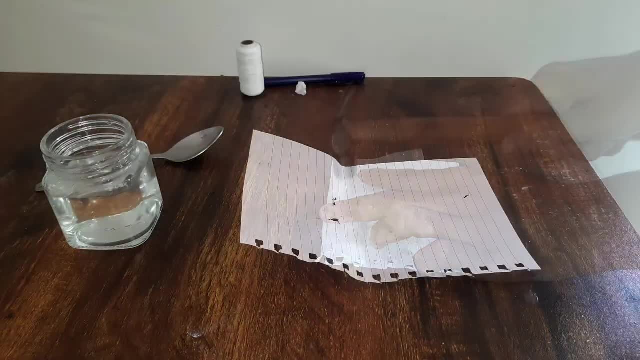 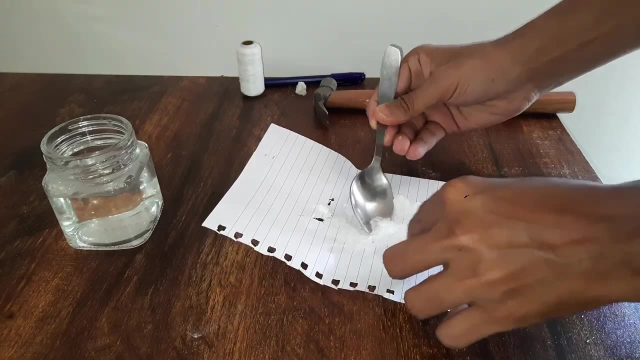 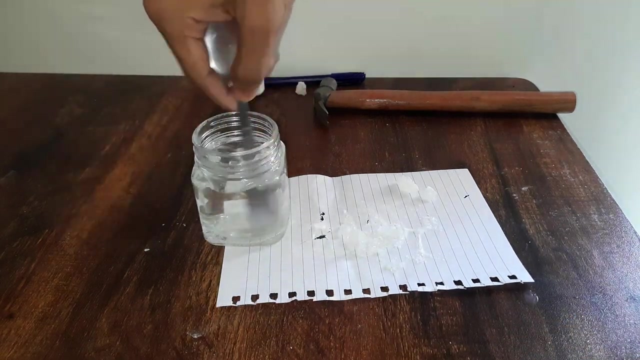 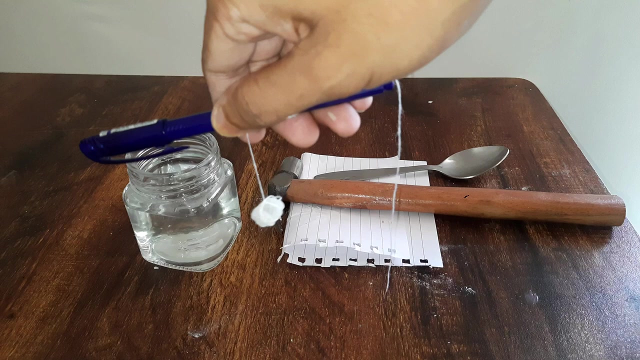 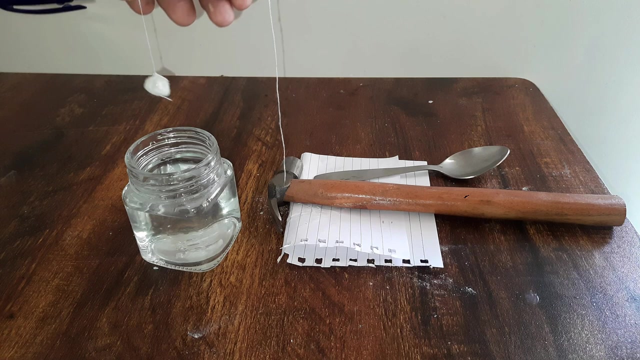 And then again try and dissolve it. So now I will add some more alum into this mixture. Alright, now what we will do is we will take one alum crystal, tie it with a string and tie the other end of the string with the pen that you see over here. 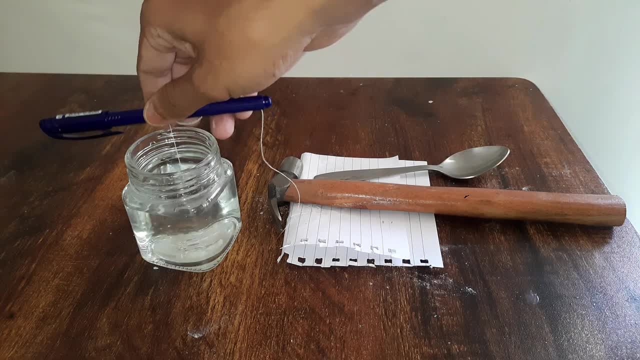 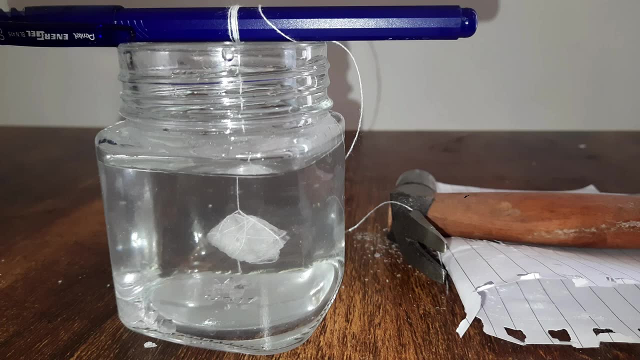 And then hang the crystal into the water like this: Make sure the crystal does not touch the base of the glass jar. We will keep it like this for at least 4 to 5 days, And now, after 4 to 5 days, let's see what happens. 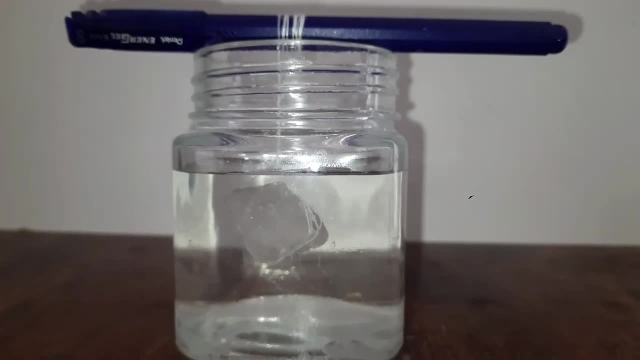 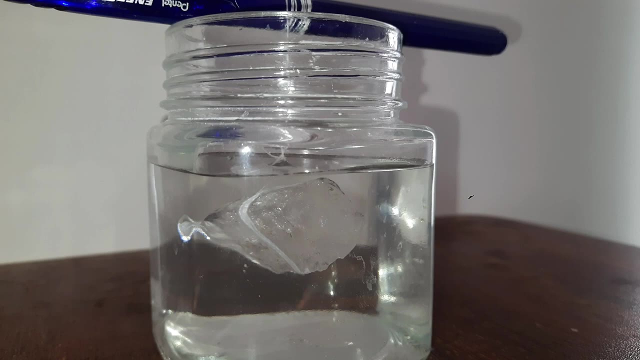 Look at the size of the crystal. hasn't it grown bigger? The size of the crystal has increased. So the question now is: is this a physical change or a chemical change? Think about it. Well turns out this is a physical change. 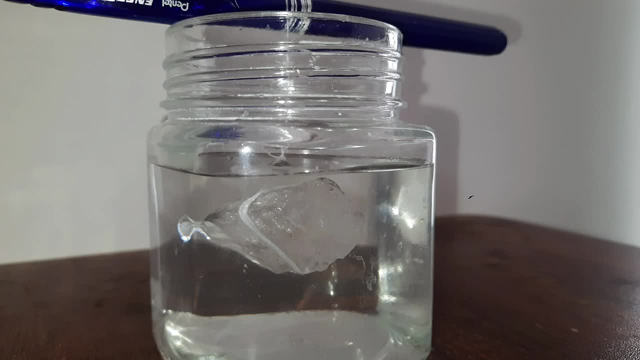 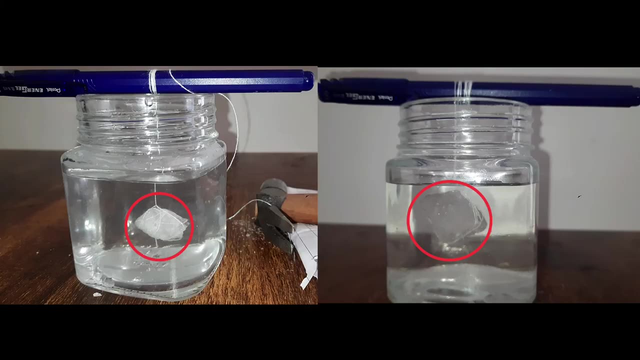 We started from alum crystals and then again. finally, we did get back all of those alum in the form of crystals. The crystal that we hung, it grew bigger. Look at the size difference in front of you. We did crush the crystals to begin with, but then we were able to obtain those crystals. 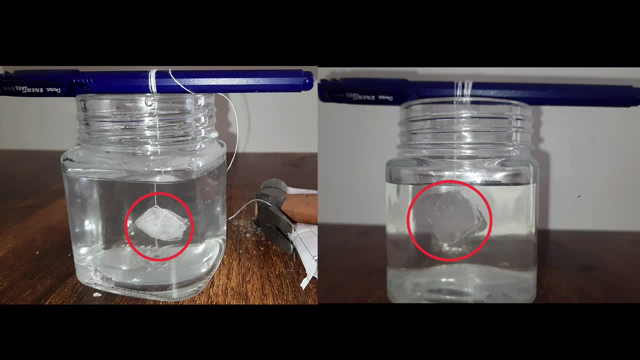 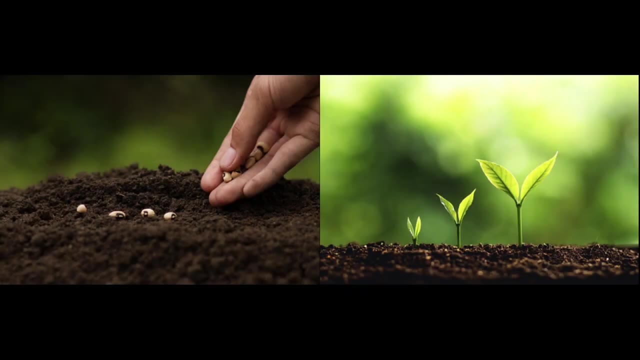 back from the water. So we started with alum crystals and we ended with alum crystals. There was no new substance that was formed, And this process, as we saw, is also reversible. So turns out, this is a physical change. Now let's look at one more example. 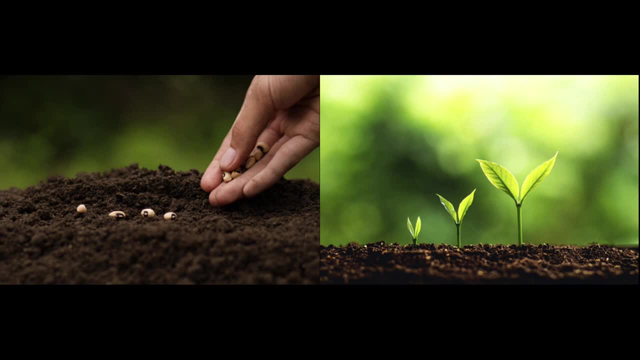 How about when you plant seeds in a soil? After some time, in fact after months, you see plants growing from those seeds, right? What kind of a change is this? Is this physical change or a chemical change? Well, turns out this is a chemical change because you can see new substances being formed. 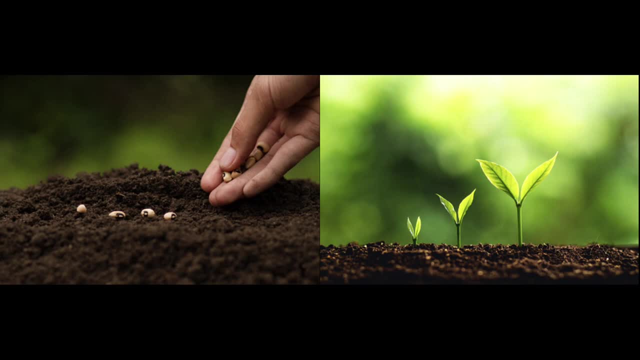 Just from seeds you're able to get a whole plant. New substances are formed, New materials are formed. You can see leaves forming, stems forming- All of these new substances are forming. and just from seed. And also once you have the plant, you cannot go back and get the seed from where it came. 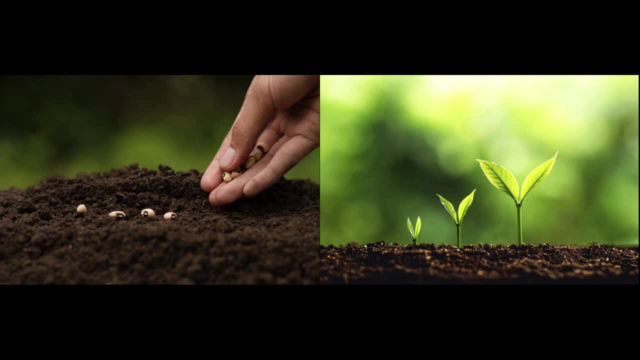 from. So turns out. growing of plant from seeds is a chemical change.